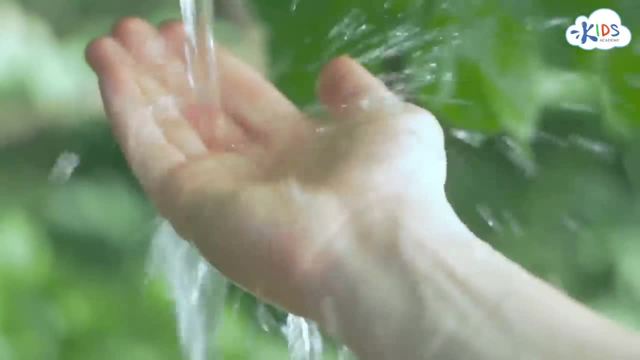 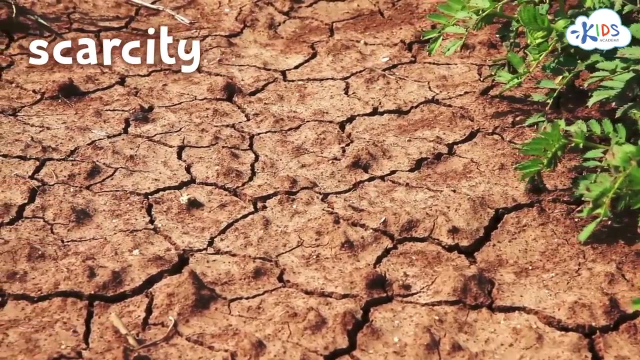 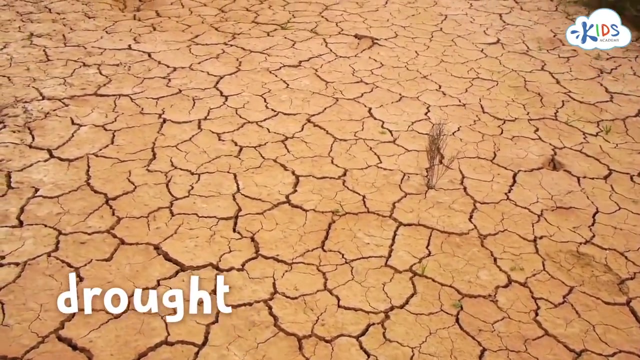 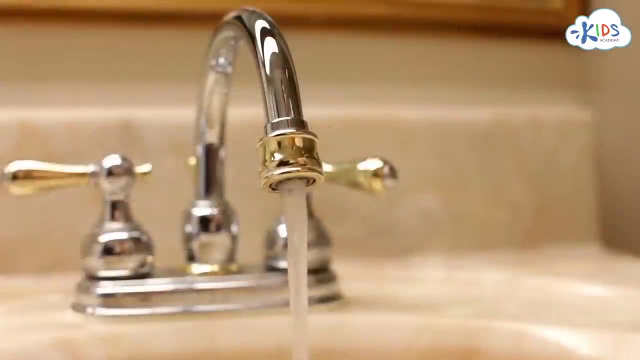 such as water and clean air. This can lead to scarcity. Scarcity is when there is not enough of something. Look at this dry land. There is not enough water to grow healthy plants. due to water scarcity, This is also called a drought. You can help prevent water scarcity by conserving. 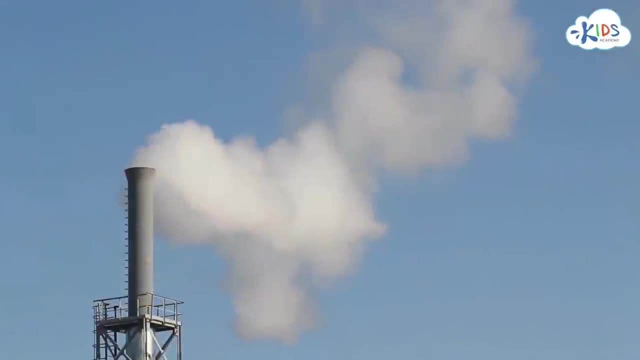 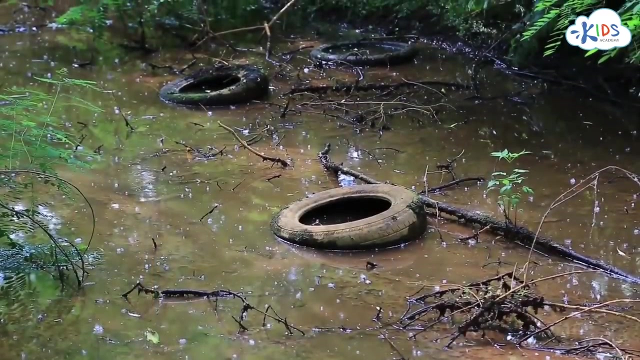 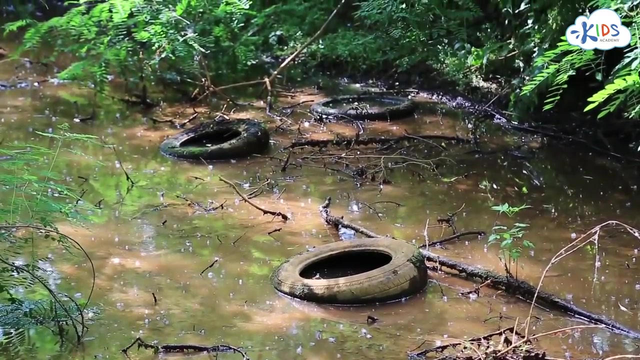 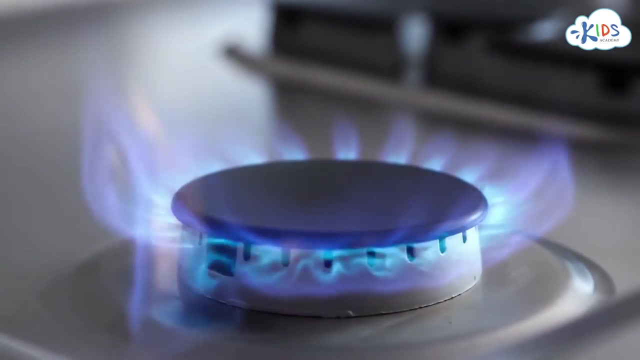 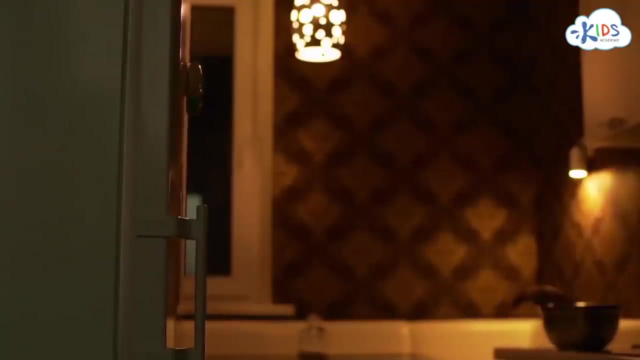 water Conservation also prevents pollution. Pollution makes our natural resources, such as air and water, dirty and dirty. We need energy, such as natural gas and electricity, to use things in our home. Televisions, stoves and refrigerators need energy in order to work Natural resources such as coal or gas. 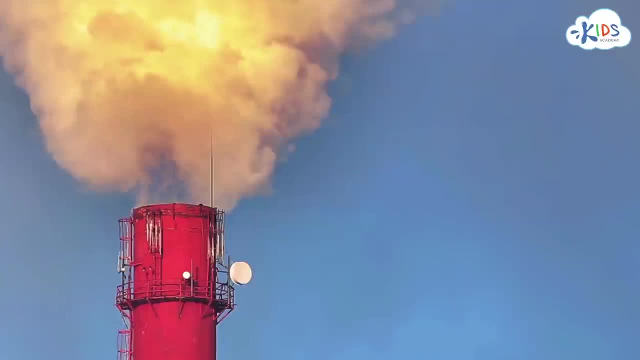 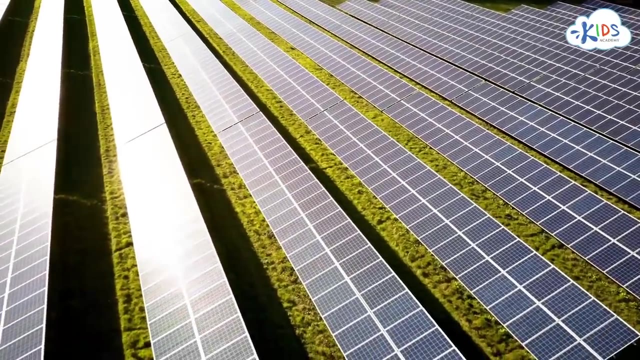 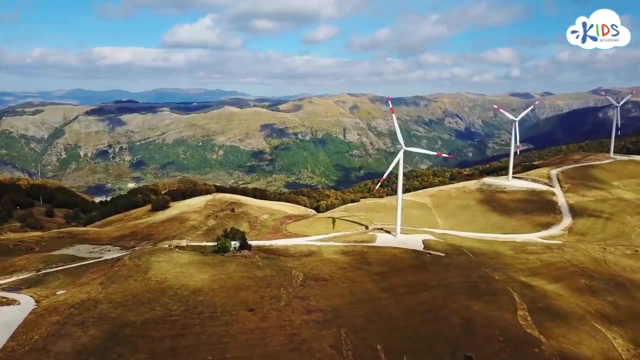 are burned in order to produce energy. The smoke spreads into the air, which can be bad for the environment. Some energy companies use solar power or energy from the sun instead. Wind power can also be used to create electricity. You can save energy by reducing the amount of electricity. 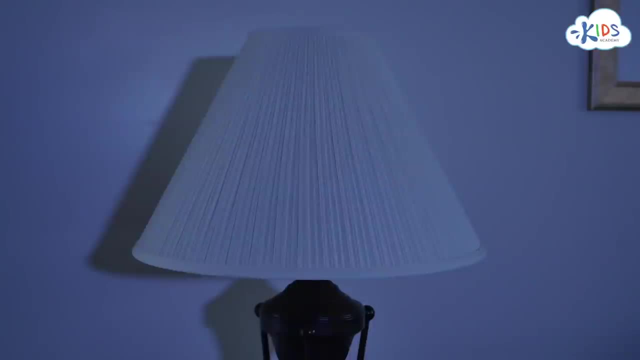 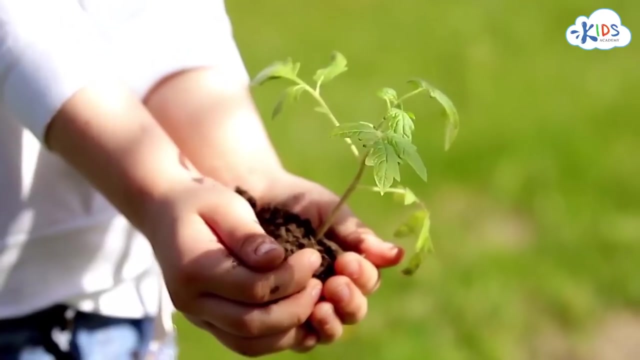 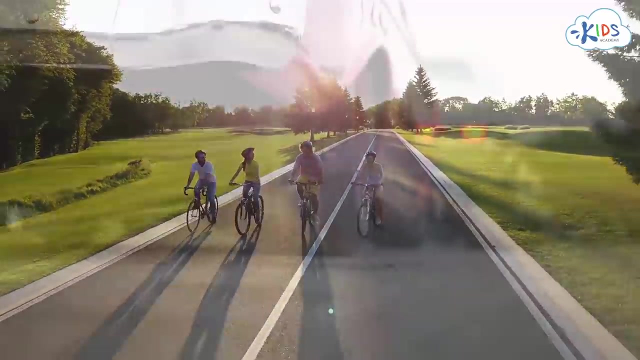 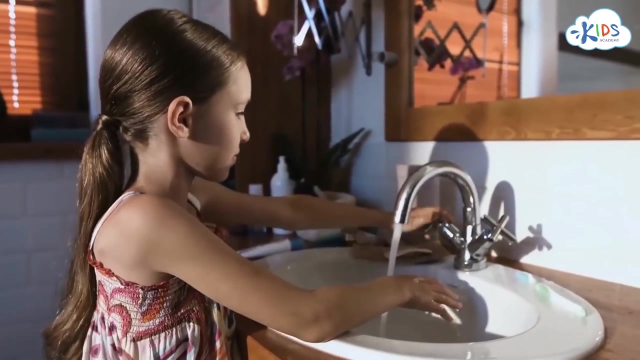 that you use. The less energy we use, the less we need to produce. So how can we conserve natural resources? Here's a few tips. Walk or ride your bike instead of riding in cars or buses. Vehicle smoke can cause pollution. Use less water. You can turn off the water while you wash your hands or brush your teeth. 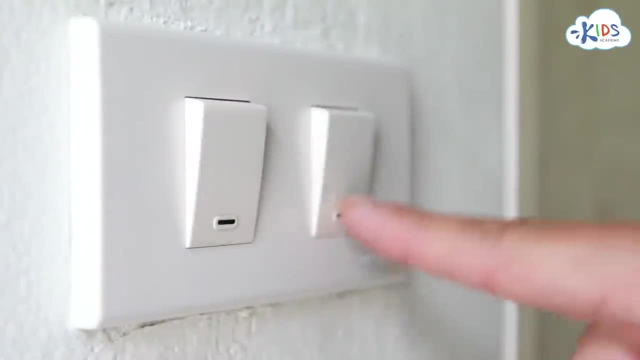 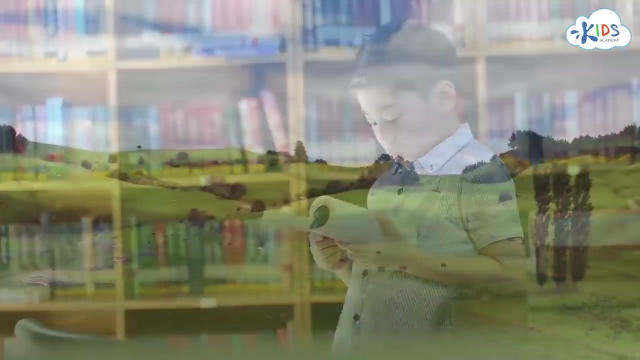 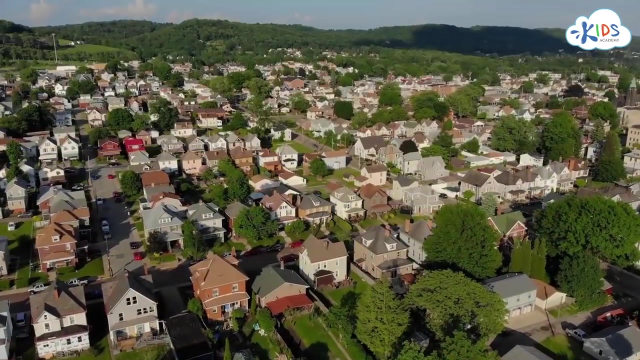 Turn off things that use electricity when you are not using them. Use sunlight instead of electric light. Together, we can protect the earth and its environment. Use resources through conservation. How can you conserve water and energy at home? Tell us in the comments below. Thanks for. 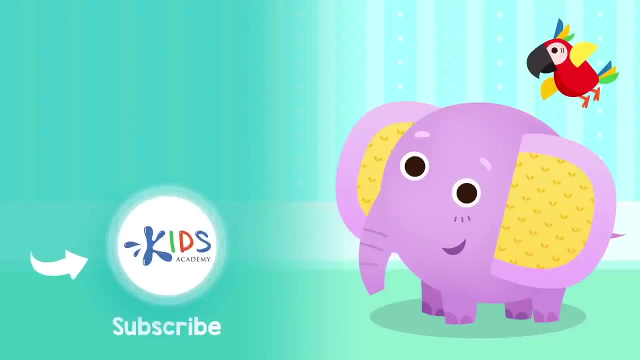 watching Goodbye. Subscribe to our channel to stay updated on new videos. Find links to our apps in the comments below.